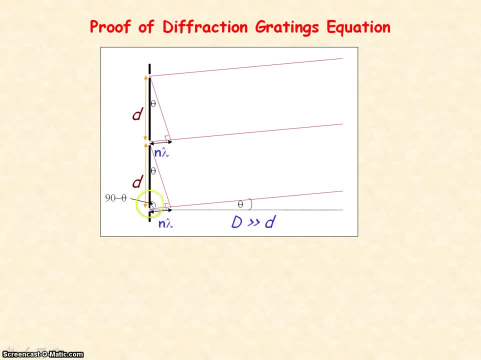 So it's for those who are interested. So here we have multiple slits Of the diffraction grating, Separated by distance d. These are representing the map waves from the slits that are meeting to form maximum n and distance d, the distance between 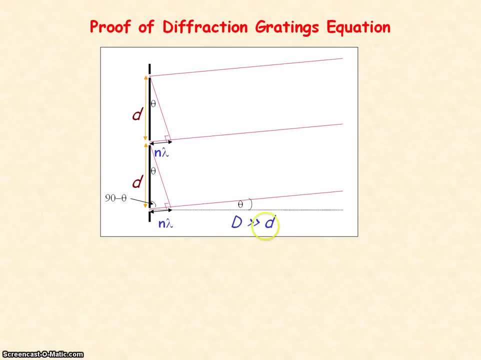 the screen and the slit is much, much greater than the distance between the adjacent slits of the grating and the light. waves are diffracted by the slit through an angle, theta. the path difference between waves from adjacent slits to reach maximum n is then n lambda. 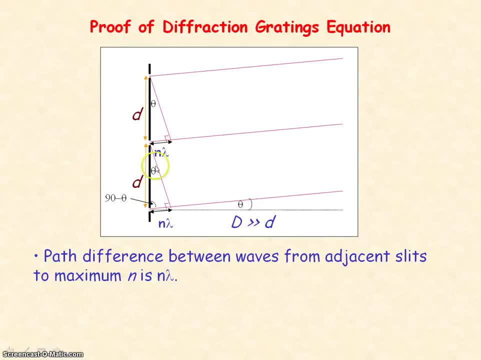 so we can use trigonometry for this right angle triangle. so relative to the angle, the path difference n lambda is opposite and distance d is the hypotenuse. so we've got opposite and the hypotenuse so we can use sine term. so sine of theta is the opposite, which is n lambda. 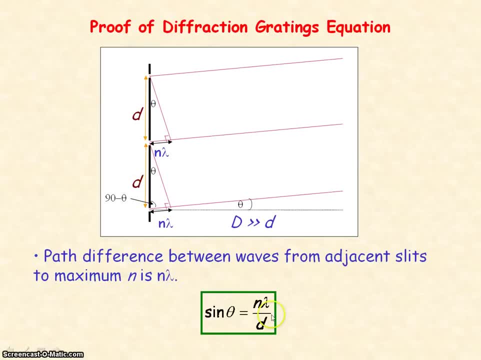 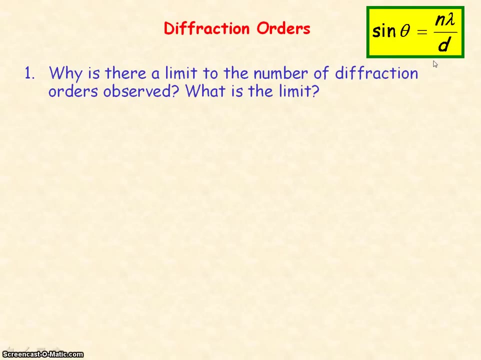 divided by the hypotenuse, which is our distance d. so remember this angle. theta is for maximum or diffraction order n. so according to this equation, there will be a limit to the number of diffraction orders observed, and that's because, sine, theta cannot be greater than one. 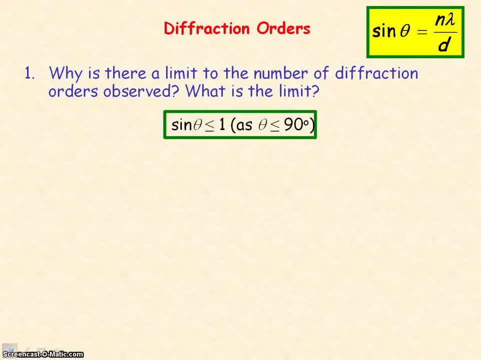 so the angle theta cannot be greater than 90 degrees. theta over 90 degrees would mean that the light waves have been reflected back off slits, which is impossible. so if sine theta cannot be greater than one, then n lambda divided by d cannot be greater than 1.. 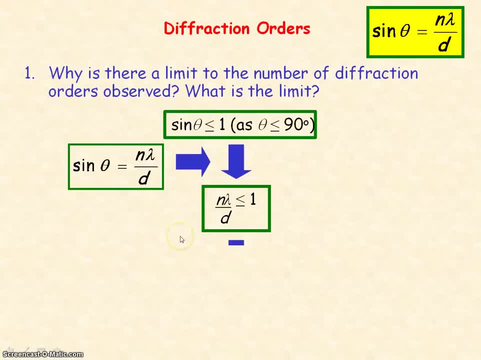 So the maximum value of n has to be less than or equal to d divided by lambda, the wavelength. So, for example, if d divided by lambda equals 4.3, as n has to be a whole number, then the maximum diffraction order observed is 4.. 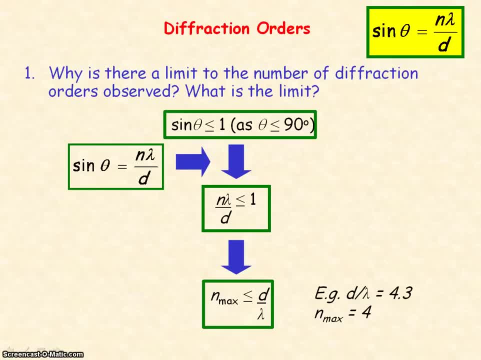 That means we'll only observe 9 maxima, the central maximum when n equals 0, and then the first, second, third and fourth maxima from both sides of the central maximum. The gratings are expressed in terms of lines per millimetre. 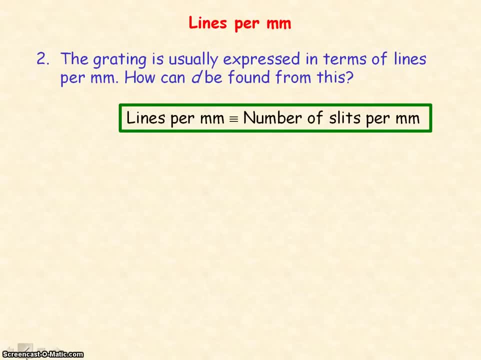 which represents the number of slits per millimetre. How we find d? d, that is, the distance between adjacent slits- is, for example, if we say we have 10 lines per millimetre, that means 10 lines occupy the distance of 1 millimetre. 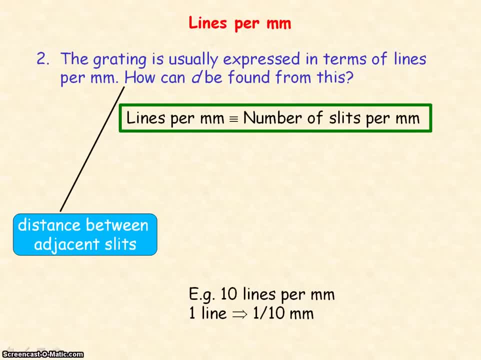 So one line will occupy a distance of 1 divided by 10 millimetres, And this then represents the distance between adjacent slits, adjacent lines, which will then be 1 divided by 10 millimetres, or 0.10 millimetres. 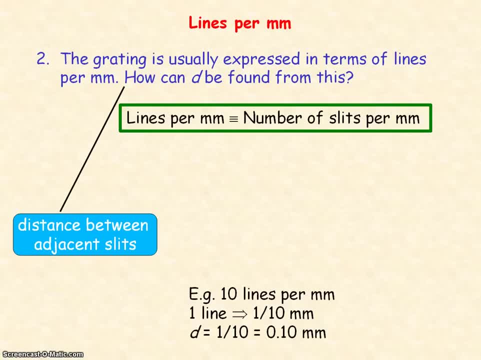 So you can see we've found d by 1 divided by the lines per millimetre, giving d in the units of millimetres. If you were given lines per metre and you did 1 divided by lines per metre, then d would be in the units of metre. 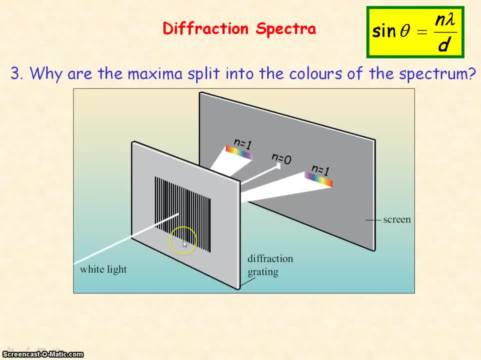 When white light is instant on a diffraction grating, then the diffraction orders will be split into the different colours of the spectrum. And that's because, as d is very small, the diffraction angle, theta, will be very big and it becomes so big that it can actually separate into the different wavelengths of light. 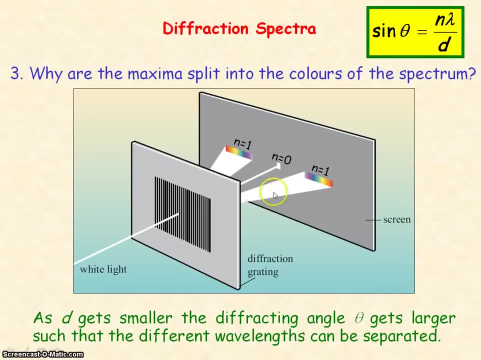 And you can see here that the diffraction angle for red light is greater than the diffraction angle for violet light And sine theta is directly proportional to the wavelength of light. So the colour of light which has a larger diffraction angle has a larger wavelength. 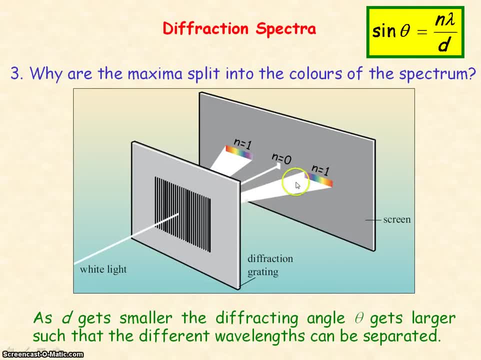 So the wavelength of red light is greater than the wavelength of violet light. It's important to note that the central maximum is white, and that's because all the colours of light reaching this point will have an overall path difference of zero. So all the colours will meet in phase and interfere constructively. 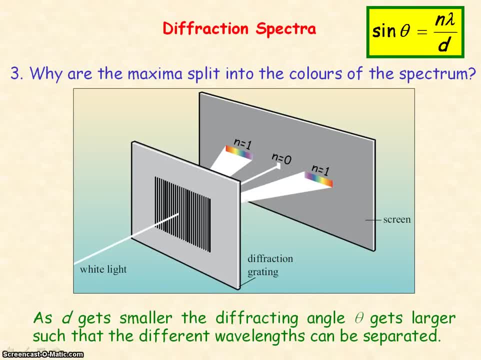 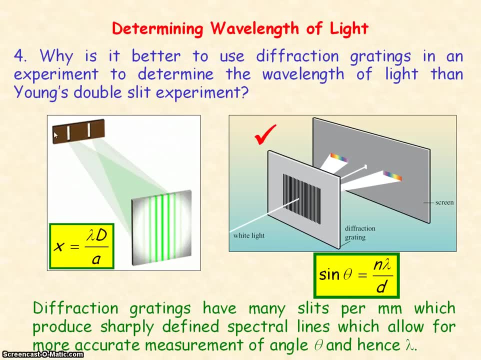 to add together to produce white light. So diffraction gratings is better to determine the wavelength of light than from the Young double slit experiment, which gave us an approximate value of the wavelength because the fringes were not sharply defined. However, diffraction gratings gave you sharply defined spectral lines. 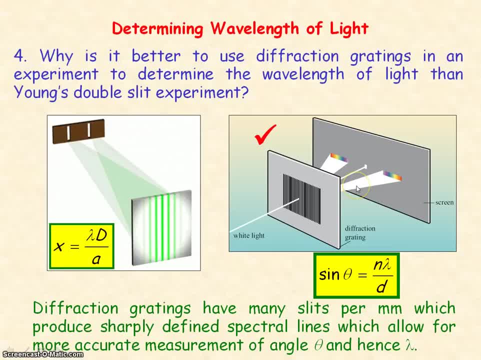 so you could make accurate measurements of the different diffraction angles of the different colours of light and hence accurately determine the different wavelengths of light for the different colors of light. so you're probably wondering: well, that's all well and good, but what else use does diffraction gratings have? well the light. 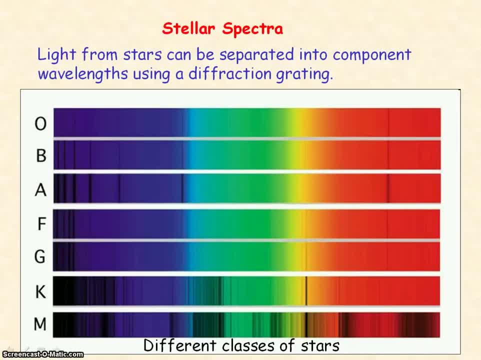 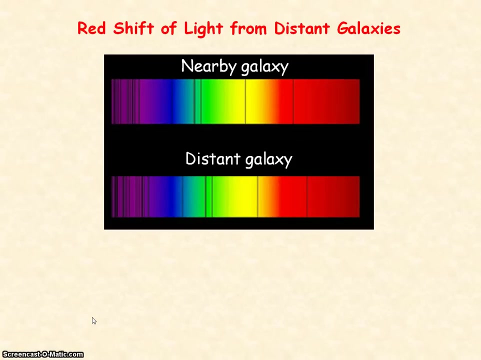 from stars and galaxies can be analyzed using a diffraction grating. so these are spectra from different types of stars, and stars are classified according to their spectrum. so the Sun is a g-type star, so the spectrum of its light would look like this. also because you could determine accurate measurements of the 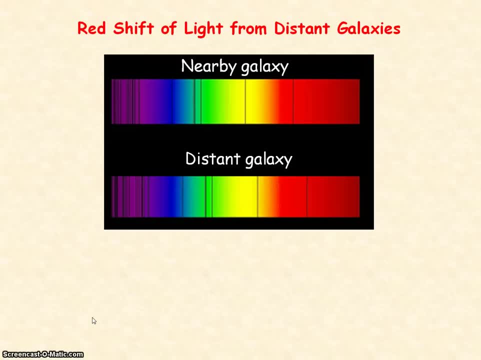 light from stars and galaxies. you could also use a diffraction grating to determine the light from stars and galaxies. you could also use a diffraction grating to determine the different wavelengths of light using a diffraction gratings. from this, astronomers were able to see.